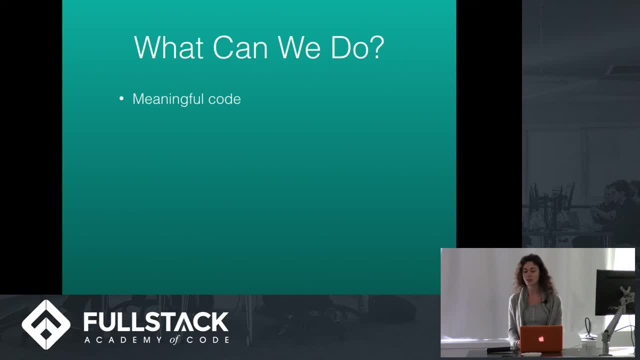 textual equivalents for images and links that are named meaningfully, And this helps with text-to-speech software as well as text-to-braille software. Then we can also facilitate users who have low vision by having content, images and text that are large or enlargeable without 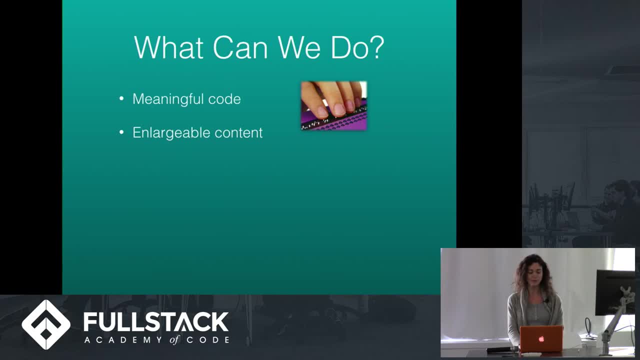 affecting the rest of the content on the page. For color deficient users, we need to differentiate color meanings. So, most notably- we see this all the time with hyperlinks- We want to signify their purpose and we see them underlined. And when you take the underline away, you need to make 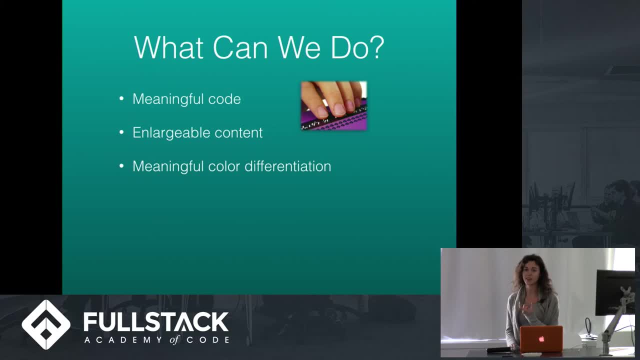 sure to signify it in some other way that it's a button or something that can be clicked for users who have color deficiency, because they might not be able to tell. Another thing we need to do for users with color deficiency is make sure to not use in tandem colors that. 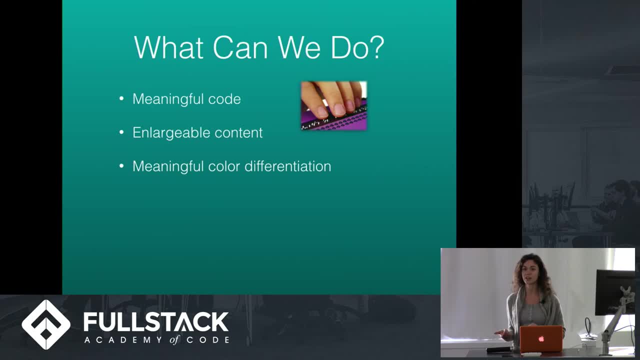 are commonly swapped, such as red and green or blue and yellow, So OK and Cancel is usually red and green. It's actually really difficult for some people because it's just gray Next to facilitate users who can't control a mouse with precision. 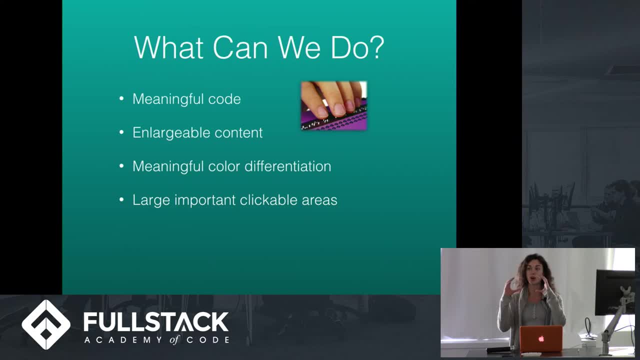 we can have important areas that are okay, have it a little bit larger And then, to facilitate users who can't use standard equipment and who need to navigate just by a keyboard or a single switch access, we make sure to include in our code something like the tab index or focus. 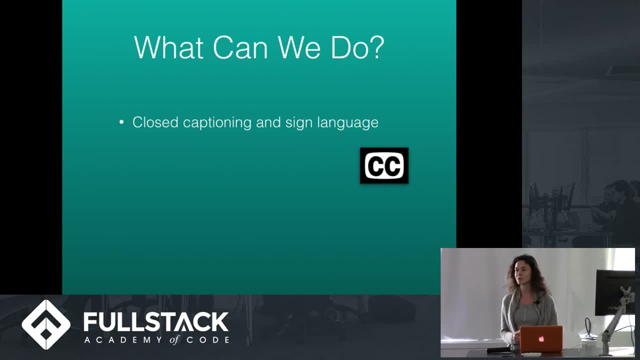 Also, we can use closed captioning or sign language versions of videos for users with auditory issues, And we can make certain effects optional, such as flashing lights. That's obviously a big one for some users. And then, finally, we can make sure to use plain language. 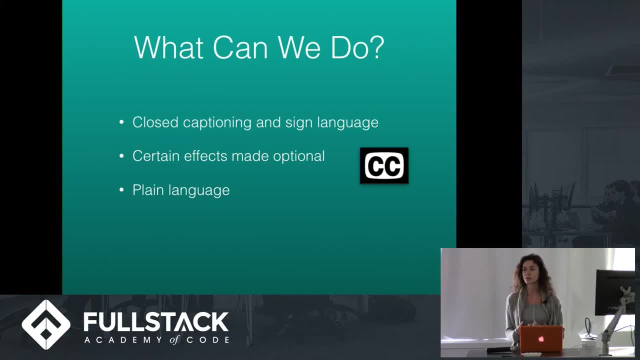 And with that also having illustrations, with instructional diagrams or animations, so that we can facilitate users with cognitive disabilities. But now that's like a list of items we can do. let's talk about the guidelines that already exist that can help us do that, as well as current legislation that you might not be aware of. 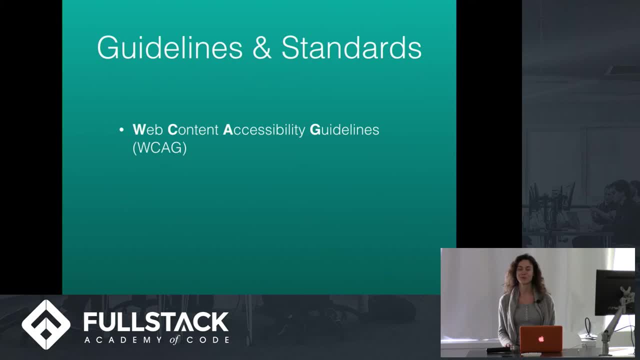 So first we have the Web Content Accessibility Guidelines created by the Web Accessibility Initiative of the World Wide Web Consortium, And they create most of the standards for all of our Internet usage. These guidelines are very in-depth and actually many policies, both public and private, are based off of them, because most governments have legislation. 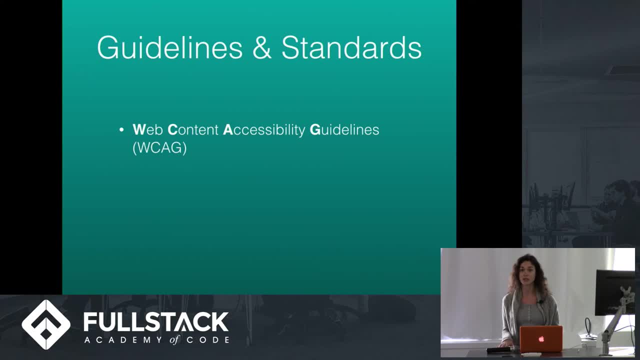 that protect disabled users' access to websites, And in the US right now these user rights are protected by the American Disability Act And there have been some notable lawsuits that actually target they. settled out of court, but it cost them like six million dollars as well as court fees. 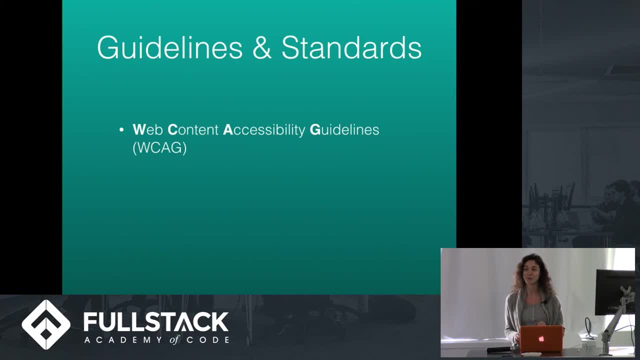 to not have an accessible website, So that's one of the things that we're trying to do. So, especially if you work at a big firm, this is important. So moving forward, we know that there's assistive technology such as screen readers. 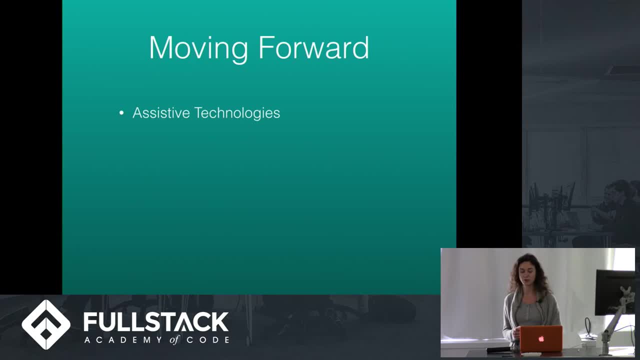 and these require semantic information to be able to process the content for users. So we need to make sure to have that semantic information. But unfortunately, as modern web applications are evolving, we're using scripts, We're applying them to our elements and making custom components, dynamic components. 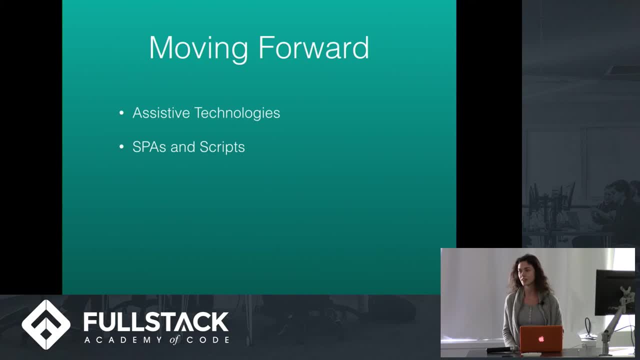 and that's yielding single page applications that most all of us are using right now. With this, HTML tags and attributes are inadequate semantic sources, as the custom components don't provide a way to have the HTML be meaningful for their state and how they relate to other elements. 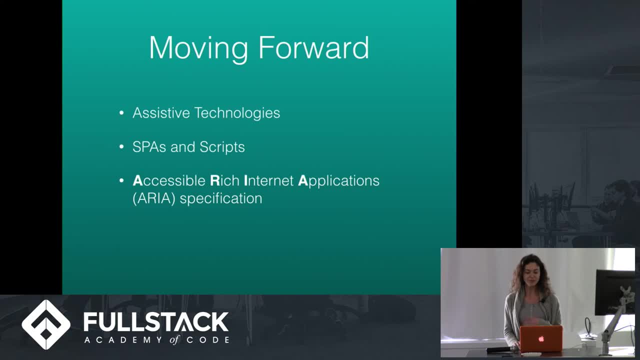 And that's what brings in ARIA. It's a specification that enables accessibility by allowing us to provide all of that information. It allows us to provide the semantics for the content that we're using. It allows us to provide the semantics for describing a dynamic component's behavior. 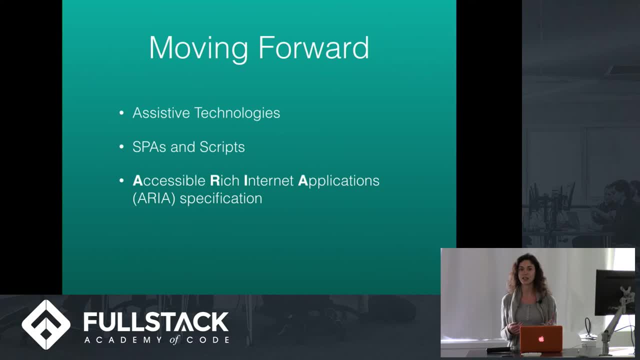 as well as by allowing us to expose a current state and how an element relates to another. And finally, the most amazing and simple way that it helps is it allows us to utilize the tab index and focus. So now here's a little. you can't see my mouse. 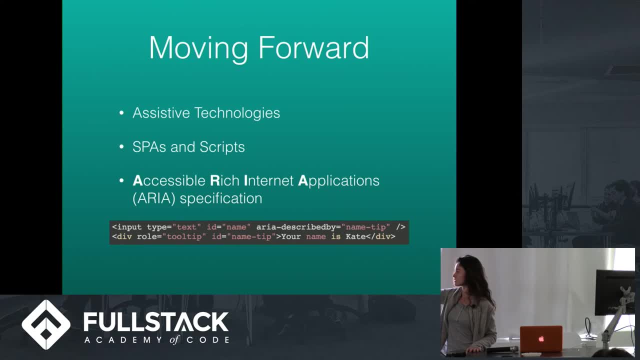 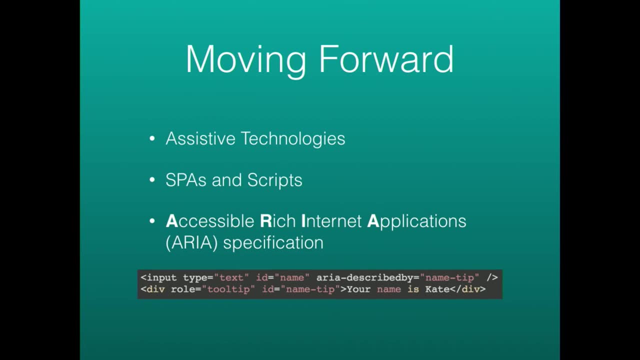 But if you look here you can see how these components- The aria-describedby is using this aria specification and it's saying: I'm described by name tip. so you know, when you find the id name tip, that these two are related, that this input is describing this div. 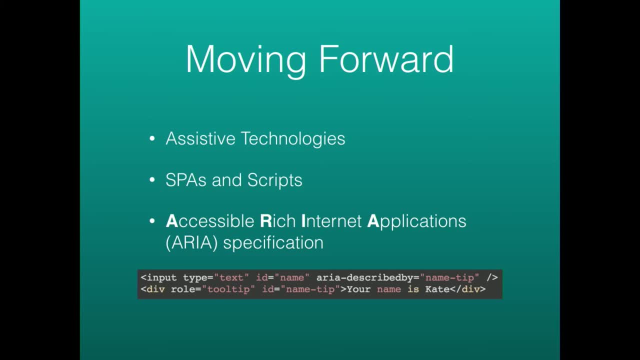 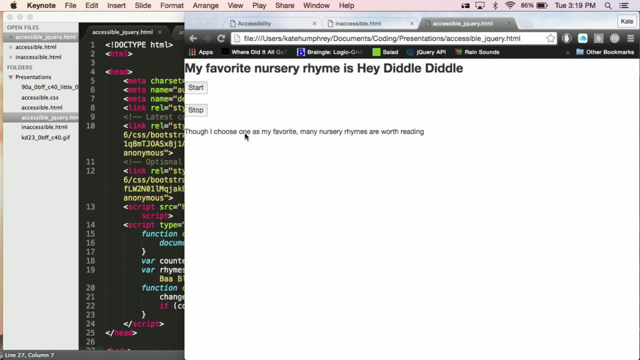 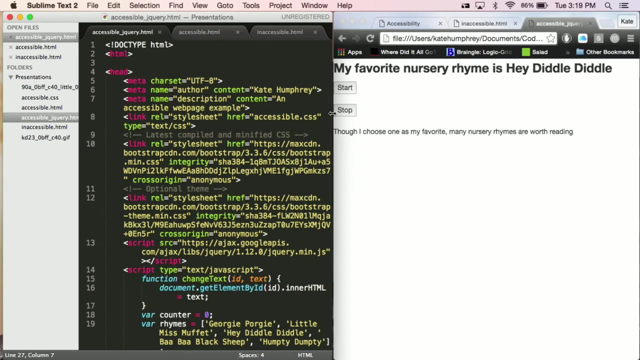 And so it's a really simple example of how they relate to each other. And now I'm going to go into an example using voiceover. It's the default on every Apple device, the default screen reader, and I'm going to just do some very basic jQuery. 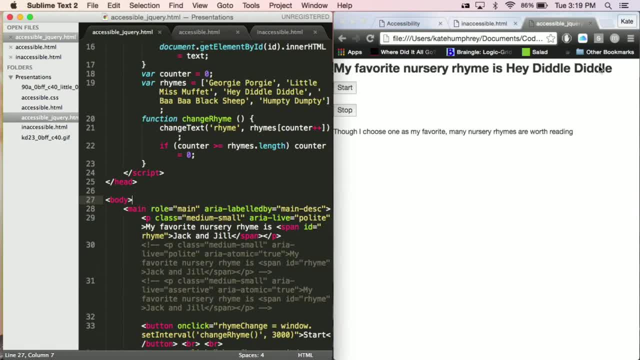 and what's going to happen is this nursery rhyme name is going to change and we're going to see how this component aria-live. It has three different states. it can be in, It can be an off, polite and assertive. and I'm just going to show you polite and assertive. 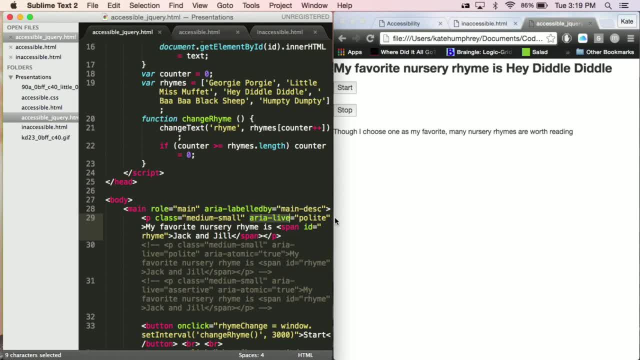 and how they differentiate and how it can really affect a blind user's access to this website. And if we have time, I'll show you a couple more examples of the screen reader. but sometimes the screen reader takes a little while, So I'm going to let it run through and I'm going to push start. 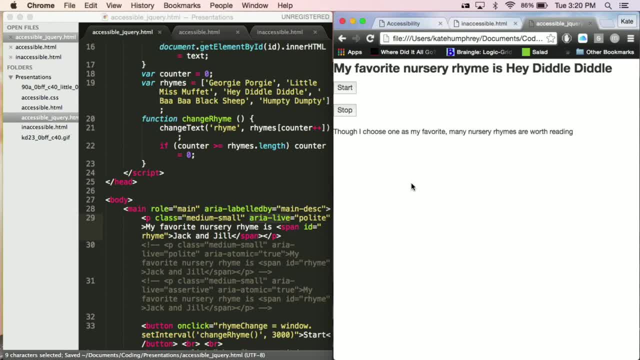 which will start changing it, And to activate voiceover, you use Command-F5.. So it should be started. I hope that we'll be able to hear it. Yeah, so I'll refresh the page So, as you can see, as you can see with aria-live, polite. 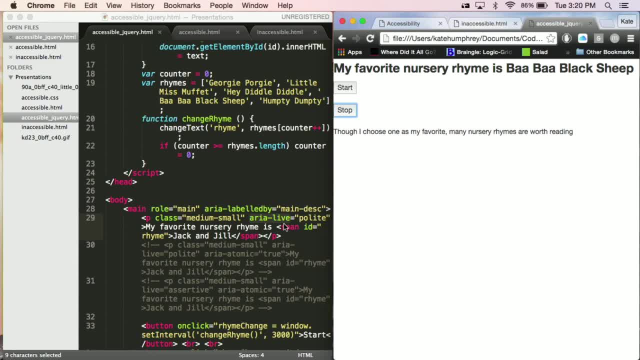 it allows the voiceover to complete reading the entire page before letting the user know that something has updated on the page. But, as you also may have noticed, it only read out the dynamic component. that did change, So I'm going to show you an alternate to this. 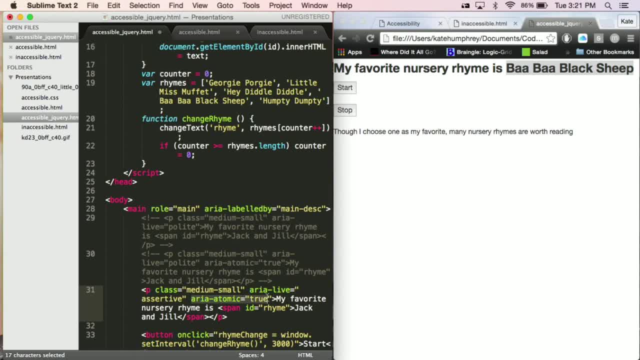 which is using aria-atomic-true. It'll read this entire paragraph element so that the user can have some context to what changed as well, as I'm just going to go ahead and show you aria-live assertive so you can see how that differs from polite. 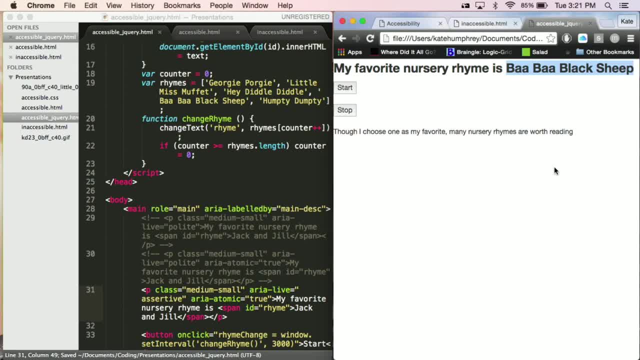 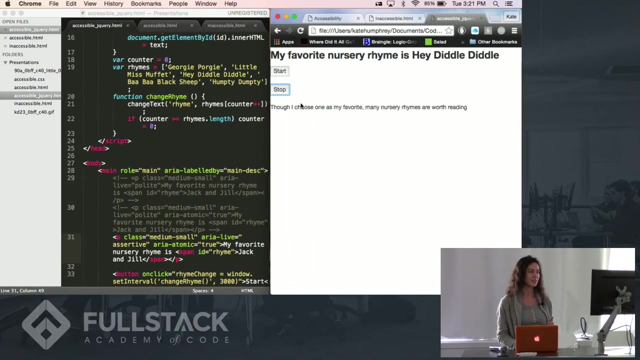 So save that and then So the difference there was that I don't know if you can really see, but it doesn't let you keep going with assertive, so that's important for when you have a warning or a pop-up. 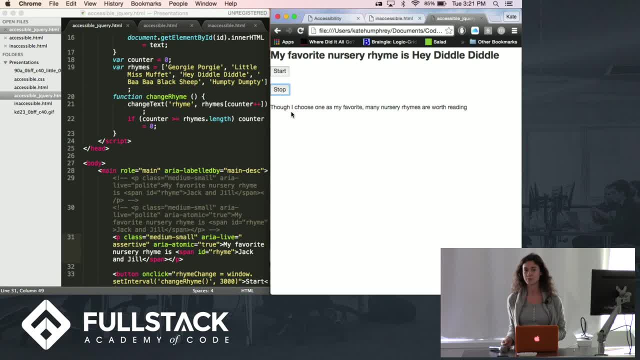 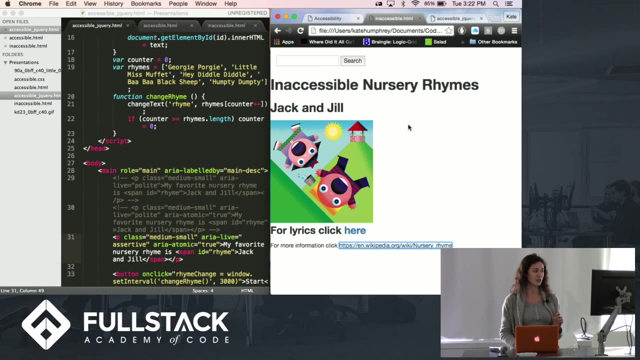 but if you misuse that, it can completely prevent certain users from being able to access your website because they're constantly just hearing that you're updating some sort of element. So if we have time, I'm going to show you a quick. This is another simple website. 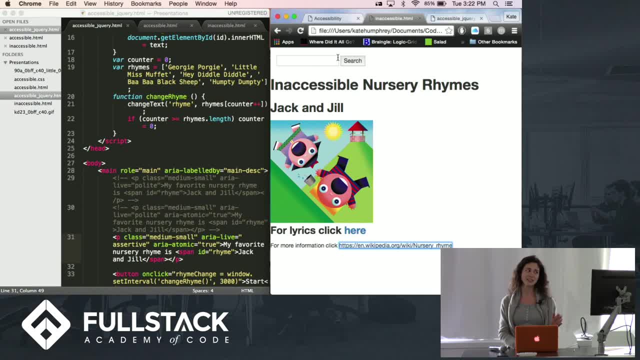 and It has a couple things that make it very difficult for users, so I'm going to go ahead and turn my voice over on Refresh the page, So it does. The first thing that was kind of problematic there was that there's just an input. 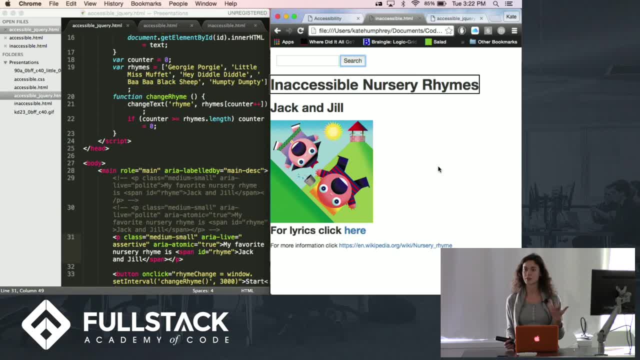 and it doesn't have any sort of context to what it does or what it is. And then further, If you don't, If you have nested HTML, you want to make sure to make it semantically meaningful so a blind user can know going into it. 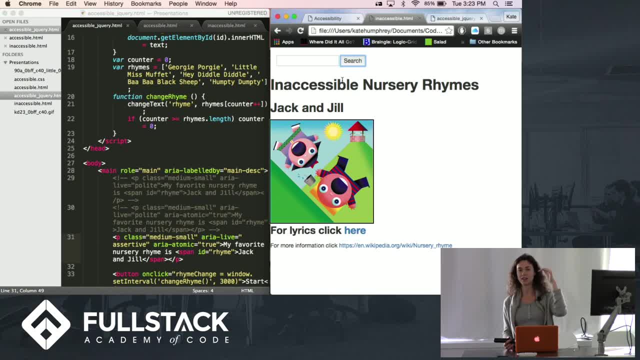 that we're on this kind of content and then we're going into it, And if you don't make that obvious in your HTML, it's very difficult for certain users And moving forward. So that's enough of that, But you see that. 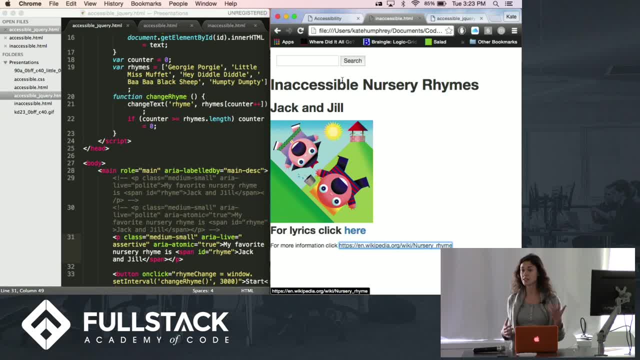 If you don't have an alternate for your image text to name it meaningfully, nobody will know, if they can't see it, what it is that they're supposed to be looking at. as well as for URLs for links, you need to have meaningful names.